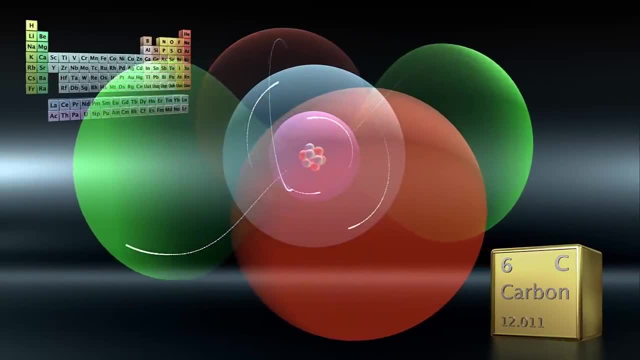 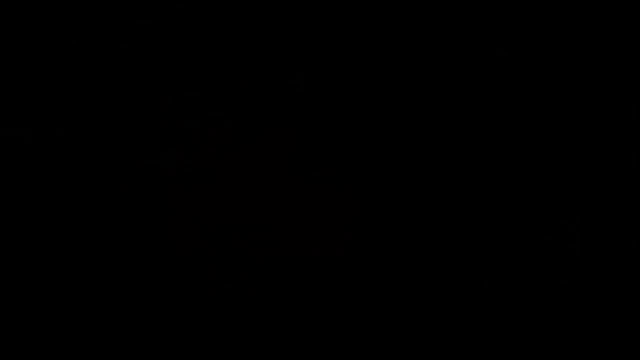 but it will be easier to keep them still in this video. We can still learn important things about atoms by simplifying the real picture. Let's pretend we have a pile of each of these particles and then build some atoms from scratch. What's the simplest and lightest atom? you? 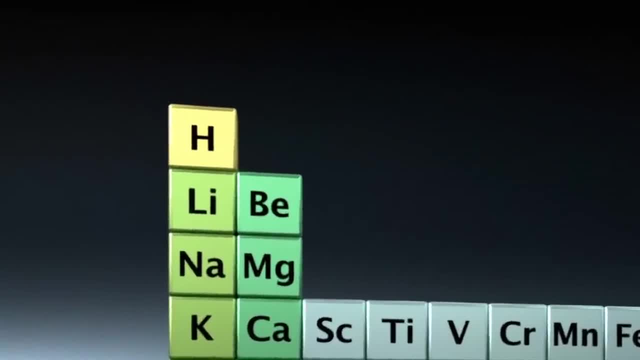 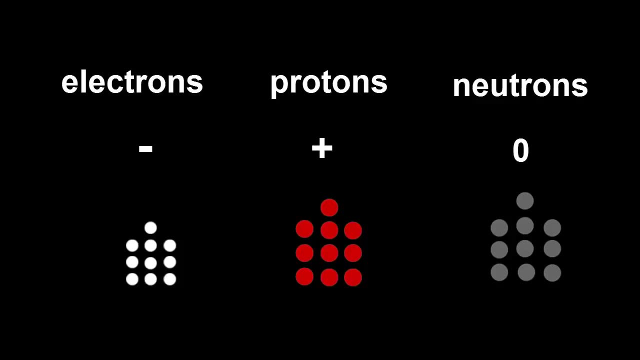 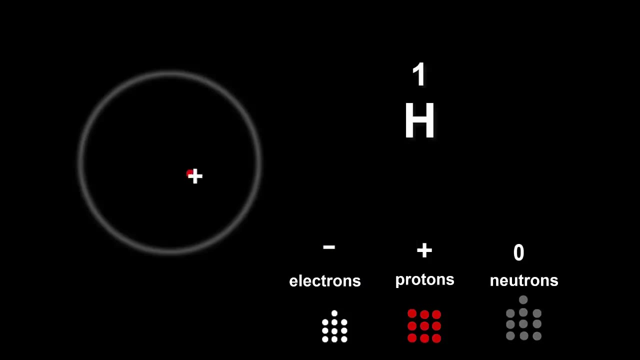 can think of, It must be the one with an atomic number of one. Did I hear you say hydrogen? It makes sense that this atom is made by using just one proton. How many electrons does a hydrogen atom need? Have you noticed that stuff around us is not? 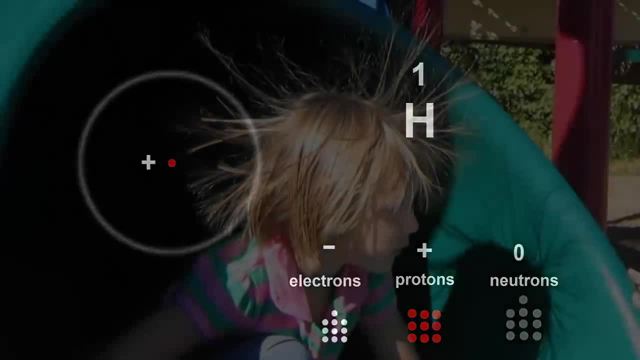 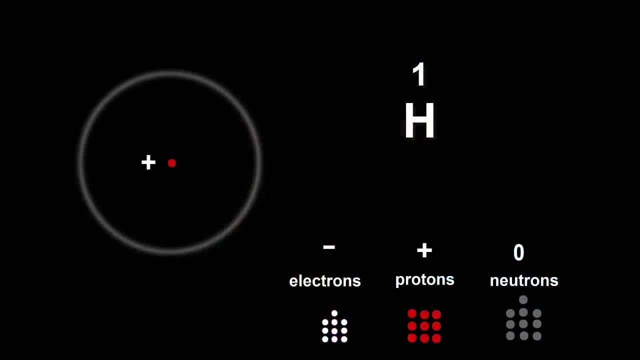 electrically charged. most of the time You don't go around with your hair standing on end from static electricity. That means that atoms are overall neutral, so that the positive charge of the proton must be exactly cancelled by the negative charge of an electron and just one electron. The number of protons and electrons must: 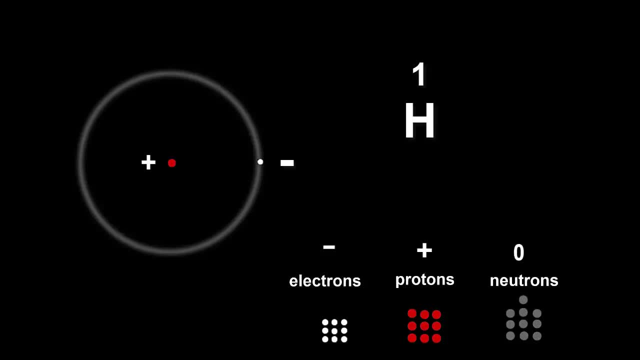 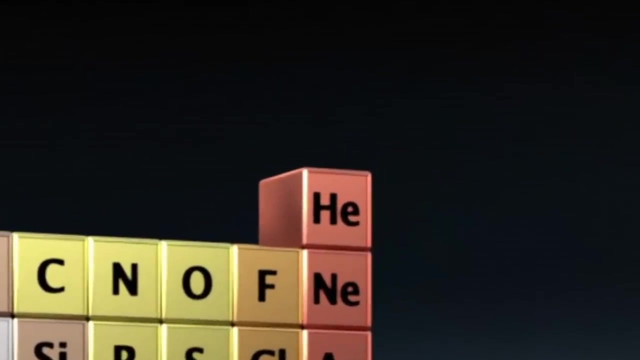 be the same. A hydrogen atom has one proton and one electron. The number of protons equals the number of electrons, And this is true for all atoms. What's the next atom on the periodic table? Helium. To make a helium atom, you need to make sure that the number of electrons is equal to the number of electrons. 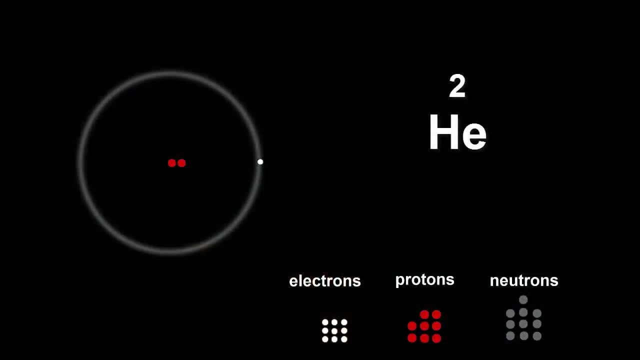 To make a helium atom, you need to make sure that the number of electrons is equal to the number of electrons. To make a helium atom, you need to make sure that the number of electrons is equal to the number of electrons. A helium atom requires two protons And how many electrons. 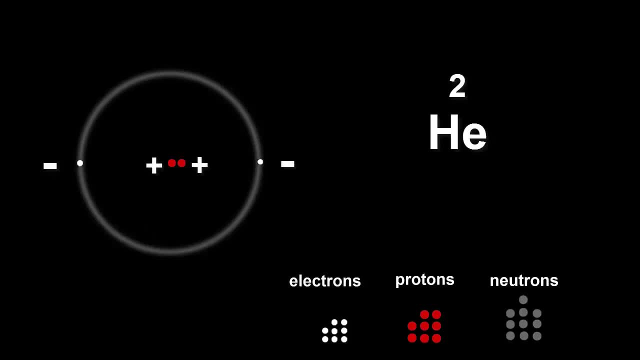 Two. We've just learnt that. Two pluses and two minuses, Overall neutral. But we have a problem, Houston. The two protons in the nucleus both carry the same charge. Why is this a problem? They will repel each other. 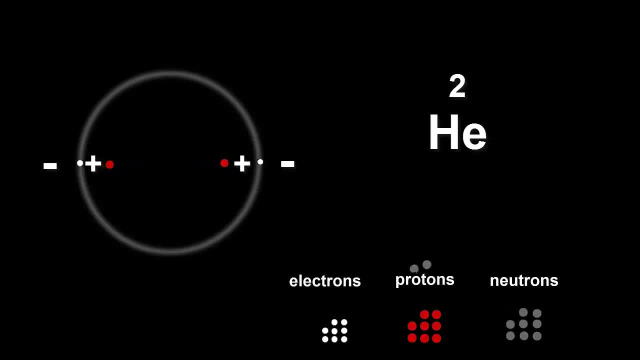 So the nucleus will fly apart. This is where neutrons come in handy. Neutrons provide some extra glue to hold the nucleus together. There's an extra attractive force that belongs in the nucleus, called the strong nuclear force. that works only between nuclear particles. 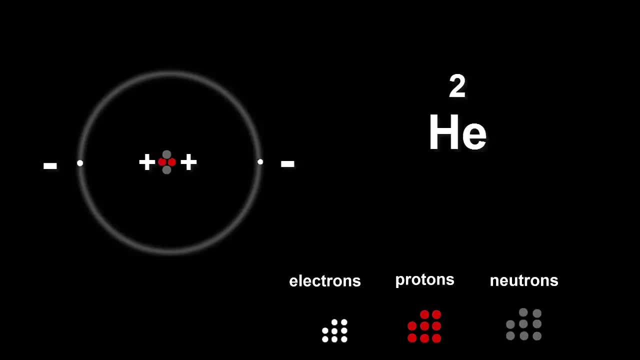 Without this force, the nucleus would disintegrate. Phew again. By the way, they won't tell you about the strong nuclear force until you get to university, So this is a kind of trailer for you. A hydrogen atom doesn't need a neutron. 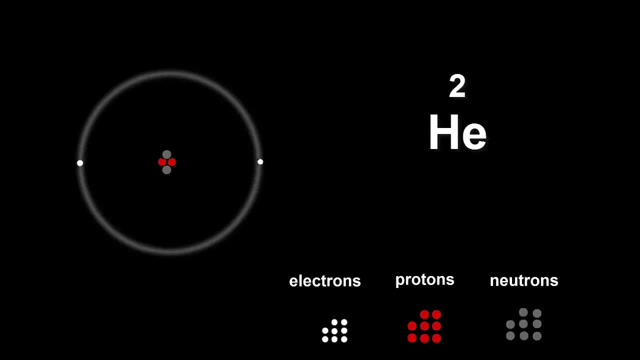 Why It has only one proton in its nucleus, so it won't fuel any repulsive forces by nearby protons. Hydrogen is the only atom that can do this. All other atoms must have neutrons in their nucleus to keep it together. 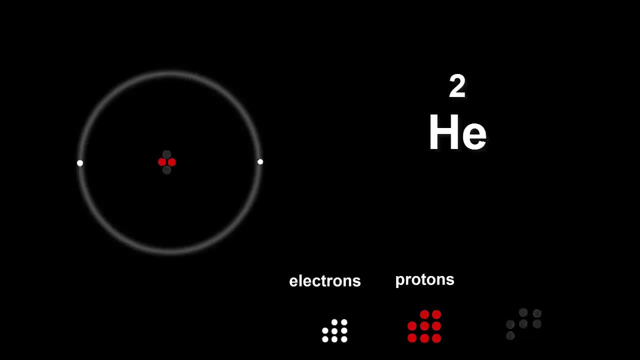 But from now on, we're going to ignore the neutrons in building our atoms to make our video easier to follow. Let's remember, though, that neutrons are found in all atoms that have more than one proton. How do we make the third atom, lithium? 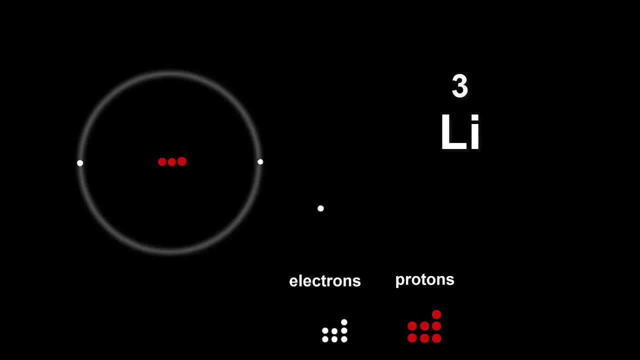 How about with three protons and three electrons? That's correct, But we've got another problem, Houston. Electrons live in shells that are wrapped around the nucleus, And the first shell can take only two electrons before it becomes full, So lithium has too many electrons. 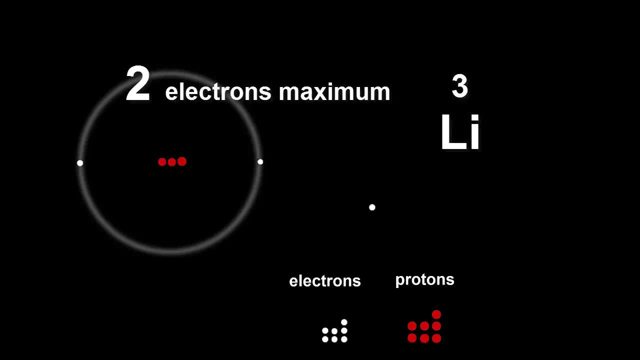 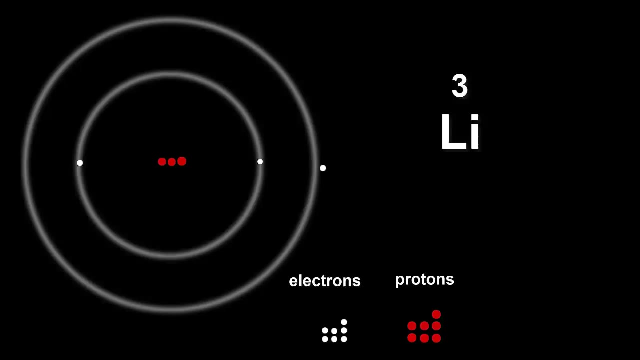 to squeeze them all into the first shell. Luckily there are plenty of shells available, So after two electrons fill the first shell, the extra electron can go into the next shell. This second shell is bigger than the first shell and can take up to eight electrons. 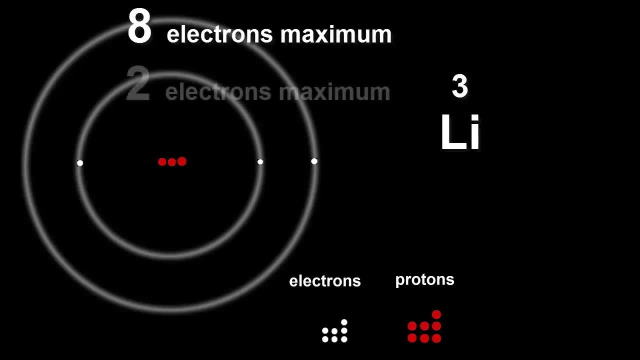 This is like a strange hotel that has only two beds on its first floor, So after two guests are booked in, extra guests have to be sent to the higher floor. The hotel's second floor has eight beds, and so after the next eight guests book in. 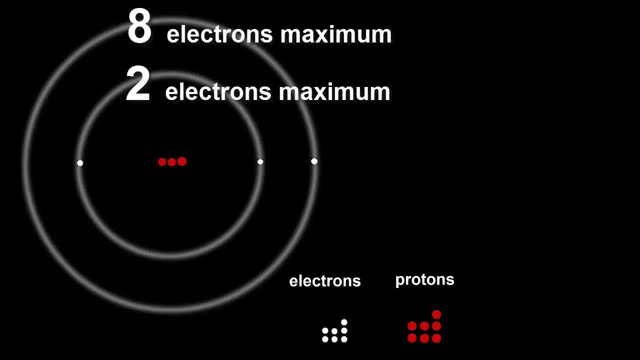 this floor is also full Since then. the number of electrons in each shell is incredibly important because it affects the properties of the element and how it will behave in the world. authorization: A lithium atom has three protons in its nucleus, two electrons in its first shell and one electron 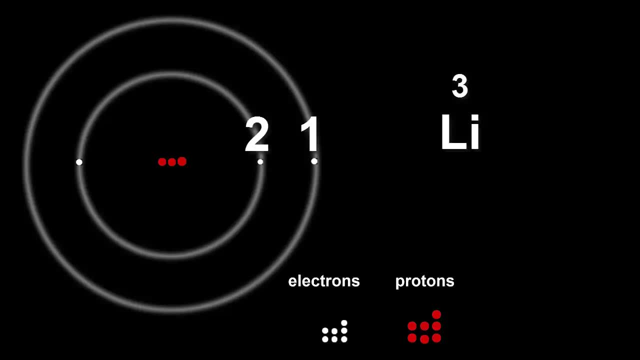 in its second shell. The number of electrons in each shell is incredibly important because it affects the properties of the element and how it will behave in the world. Here is a simple example. Here is a picture of a rare electron world. For example, lithium is a metal because it has a single electron in its outer shell. 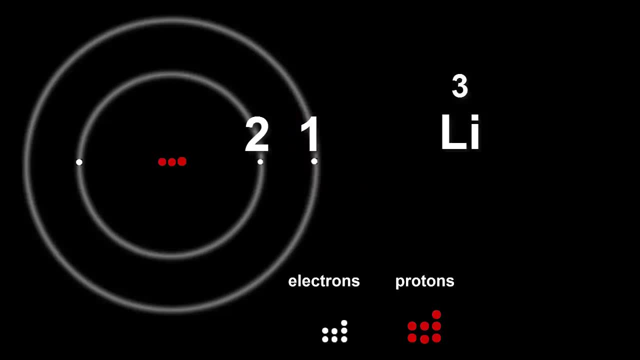 We will explain how this happens later. The number of electrons in each shell of an atom is called its electron configuration. You should ask your parents if they know what electron configuration means. They're really cool words to learn. The electron configuration of lithium is 2 electrons in the first shell and 1 electron in the second shell, Or sometimes. 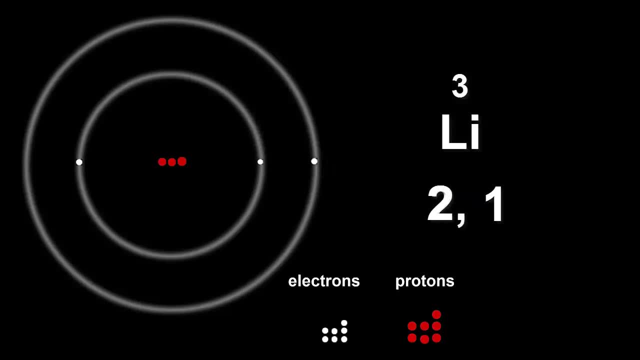 scientists just write 2,1 for short. We're on a roll here. What is atom number 4 and how many protons and electrons does it have and where do they live? Did you say beryllium with 4 protons and 4 electrons, With all 4 protons living in its nucleus, 2 electrons? 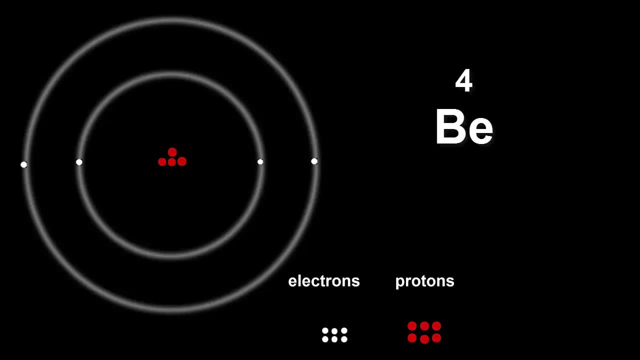 in its first shell and 2 in its second shell. If so, you can move to grade 11 in high school. Beryllium's electron configuration is 2,2.. 2 electrons in the first shell and 2 electrons in the second shell. 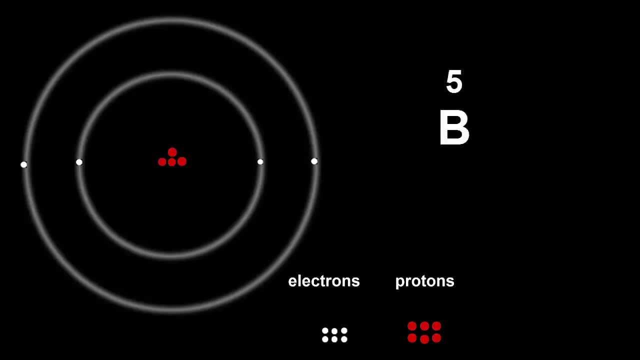 Next atom is number 5, boron. It has 5 protons and 5 electrons: 2 electrons in its first shell and 3 electrons in its second shell. Its electron configuration is 2,3.. Then number 6, carbon: 6 protons and 6 electrons. Its electron configuration is 2,2.. 2 electrons: 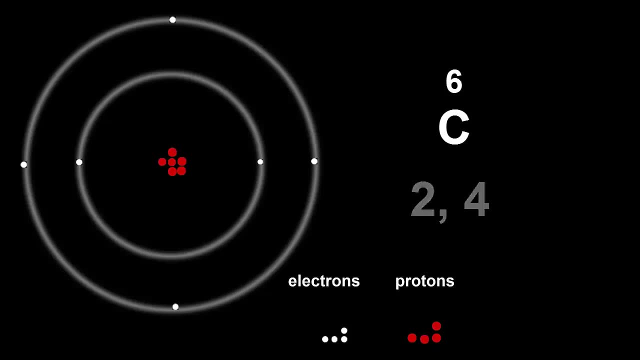 in the first shell and 3 electrons in its second shell. The electron configuration is 2,1.. De fitted in baltimore to 1 ox blah ya, 0 ox blah 4.. At the moment I'm going to quick go through this previous example here. 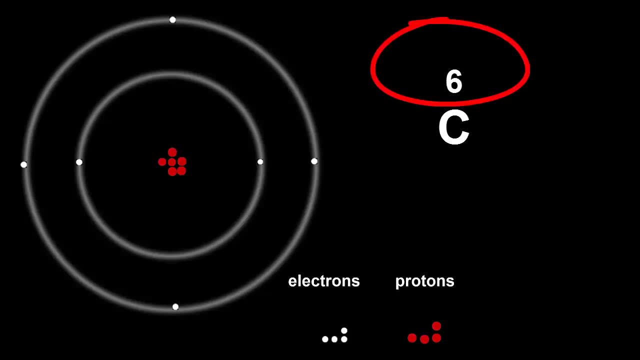 But I�m going to do that next time because maybe I'll make a follow-up to it. that's better recording for you later. Did you notice a pattern here? The number of the atom is always the same as the number of protons in its nucleus. Earlier we learnt that atomic number meant. 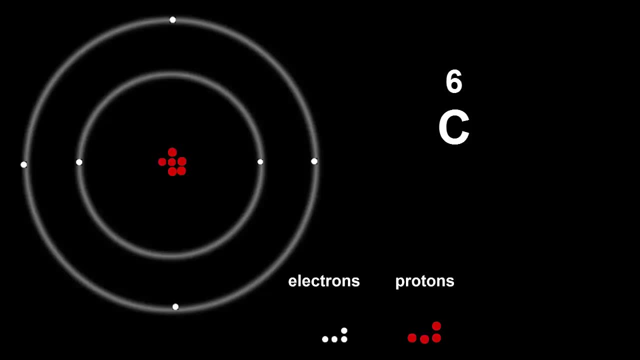 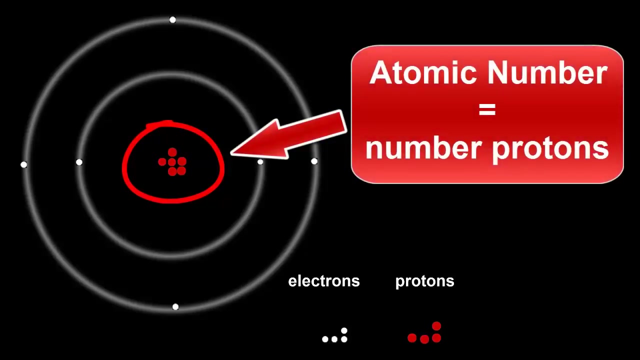 the place of an atom in the list of atoms from the lightest to the heaviest. When scientists discovered these sub-atomic particles, they realised that atomic number was also exactly was also exactly equal to the number of protons in the nucleus. It means that an atom's identity, that is, whether it is hydrogen or aluminium or gold. 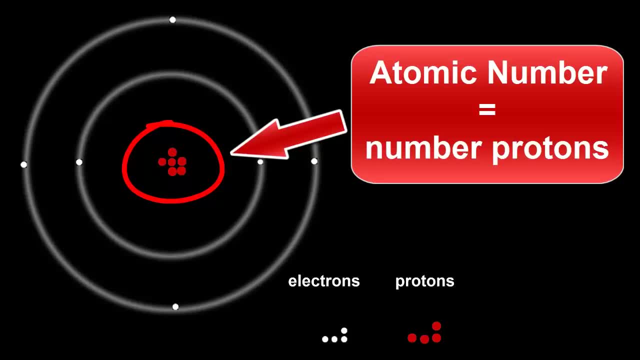 depends only on how many protons are in its nucleus. The atomic number of an atom is equal to the number of protons in its nucleus. We could have defined the atomic number as the number of electrons, as this is the same as the number of protons in an atom. 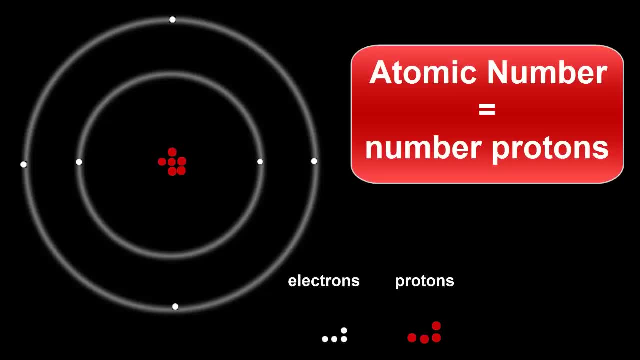 However, electrons can sometimes be swiped off the outside shell of an atom, or an atom may grab an extra electron or two. So this is the atomic number. This number of electrons can vary from time to time. Protons live in the nucleus, which is locked away from the outside world. 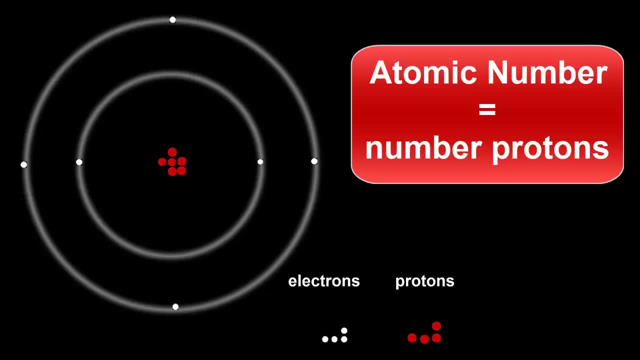 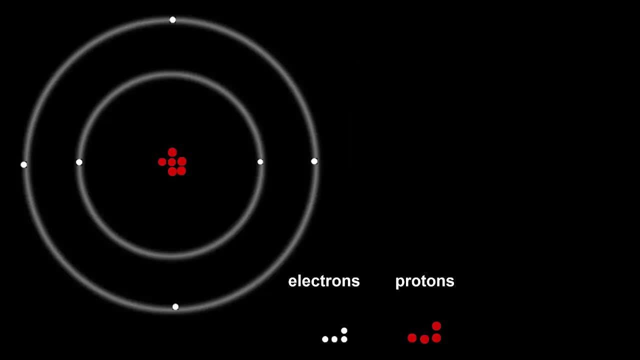 and their numbers don't vary usually. This is a better definition. Let's use up the rest of our protons and electrons. Number seven: nitrogen: Seven protons and seven electrons. Electron configuration: two: five: Two electrons in the first shell and five in the second shell. 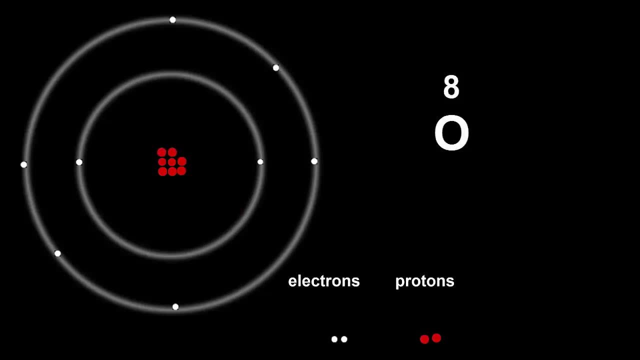 Number eight: oxygen. Eight protons and eight electrons. Electron configuration two- six. Two electrons in the first shell and six in the second shell. Number nine: fluorine. Nine protons and nine electrons. Electron configuration two- seven. 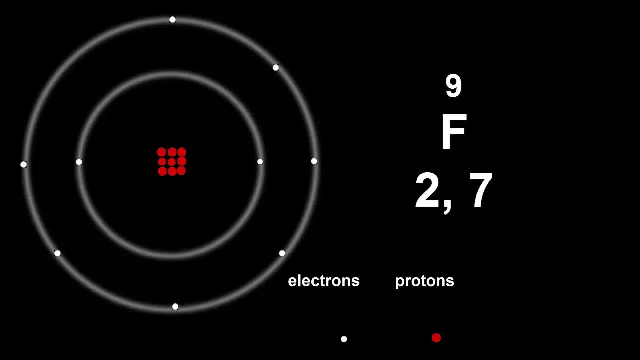 Two electrons in the first shell and seven in the second shell. Number ten: neon, Ten protons and ten electrons. Electron configuration: two: eight. Two electrons in the first shell and eight in the second shell. Remember how many electrons that the second shell contains.